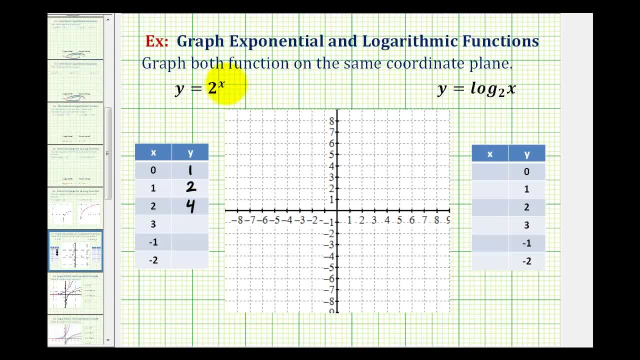 When x is three, y is equal to two, to the third equal to eight. Notice I also selected two negative values for x. When x is equal to x, negative one we would have: y equals two raised to the power of negative one, which would be: 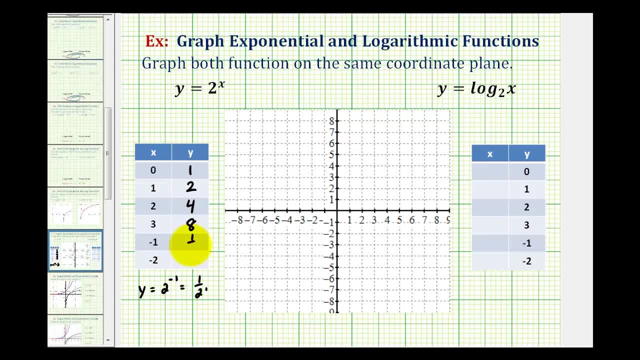 one over two to the first, or just 1: 1⁄2.. When x is negative two, y is equal to two to the negative two, which is equal to one over two squared, which would be 1⁄4.. 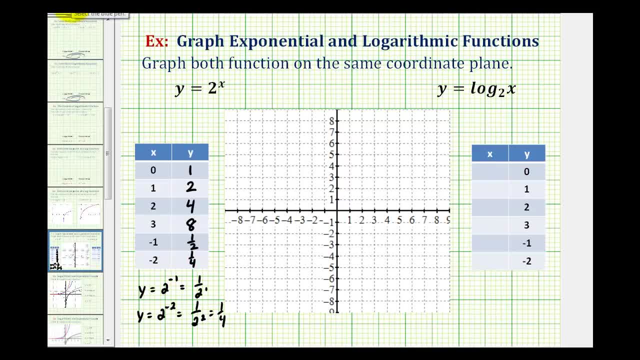 Let's go ahead and plot these points on the coordinate plane and sketch our graph, And we'll sketch the exponential function in blue. So we have the point zero one, which is the y-intercept. We have the point one, two. 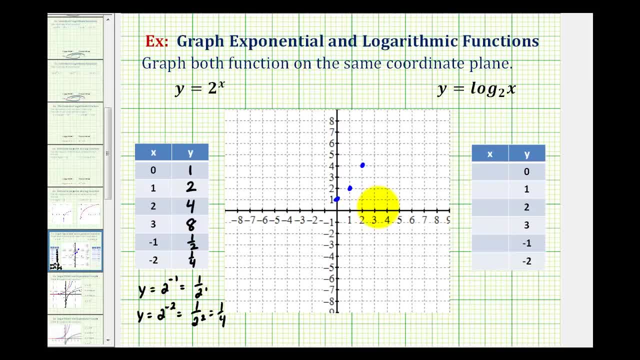 Point two, four, Point three: eight: Negative one, 1 1⁄2,, which would be here, And negative two 1⁄4,, which would be here. So our function looks something like this: Notice how we have exponential growth. 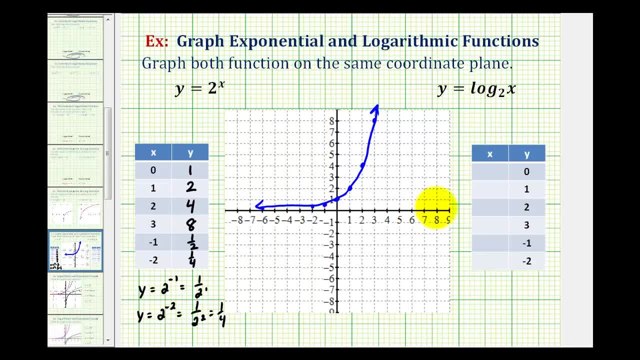 because the function is the base is greater than one. We have a horizontal asymptote along the x-axis, or y equals zero. Notice the domain or all possible values. of x would be all real numbers, But the range or the y values would be. 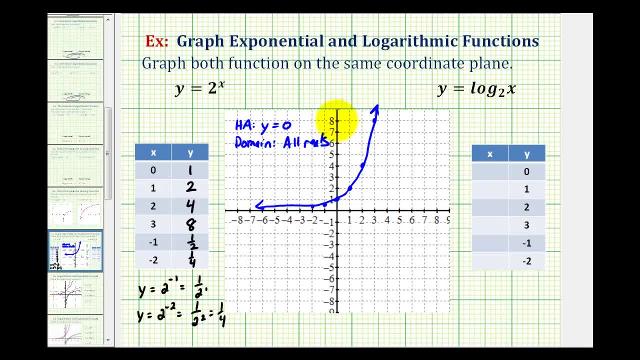 y is always greater than zero because the function is always above the x-axis And the lesser the number, the average. Now to sketch the log function, we're going to rewrite this in exponential form. number y equals log base. two of x is equivalent to two raised to the power of y. 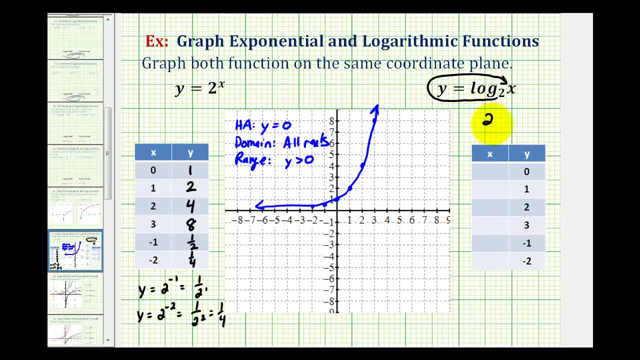 must equal x. So to complete a table of values for a log function, it's easier to rewrite it as an exponential function. Then, instead of selecting x values, we select y values to determine the value of x. But before we do this, notice this equation here. 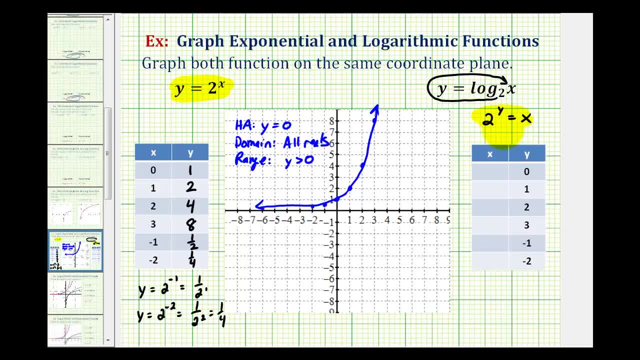 and this equation here look very similar, except the x and y variables have been interchanged. So because y is now the exponent, we'll select y values and determine x. Notice how these y values here are the same as the x values we had here for the exponential function. 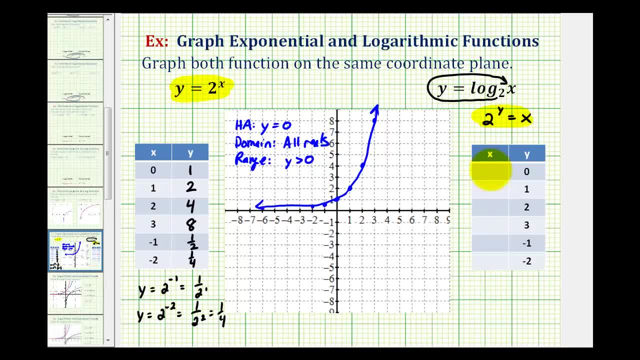 So when y is equal to zero, we have two to the zero equals x, so x is one. When y is one, two to the first equals x, which is two. When y is two, two squared x would be four. 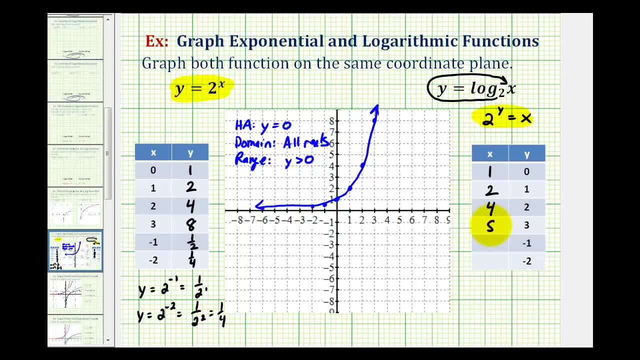 When y is three, two to the third equals x, or eight equals x. When y equals negative one, we'd have two to the negative. one equals x, which is one half, And when y is negative two, we'd have y to the negative two. 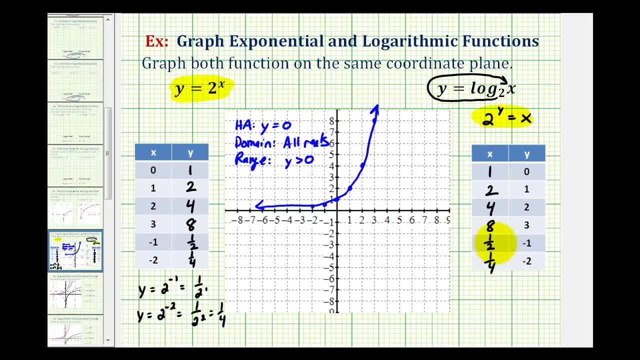 equals x, which is one. fourth. Now let's go ahead and sketch the log function in red. So we have the point one zero, we have the x-intercept two, one, four, two and eight, three, As well as one half negative one. 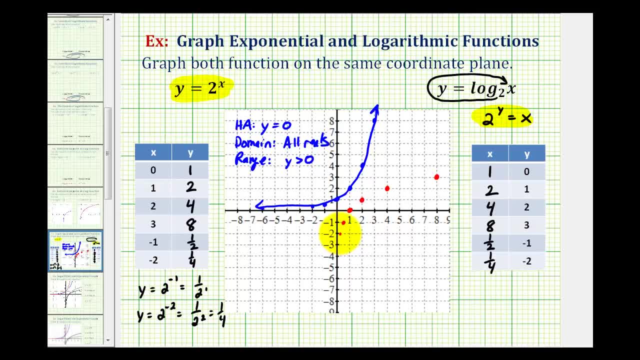 and one. fourth negative two. So our log function looks something like this. Now, there are several things to notice about this function. The log function has a vertical assin tot, which would be the y-axis. with a vertical line, x equals zero. 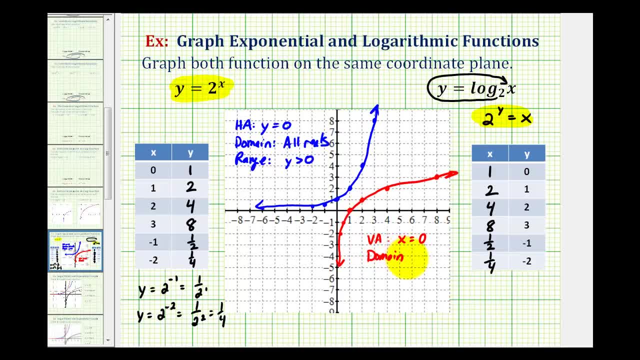 Notice, the domain of this function would be x greater than zero And the range of this function would actually be all reals, because this function goes down forever as well as goes up forever. Now, if we compare these two functions, notice how, looking at the table of values, notice how the x and y coordinates. 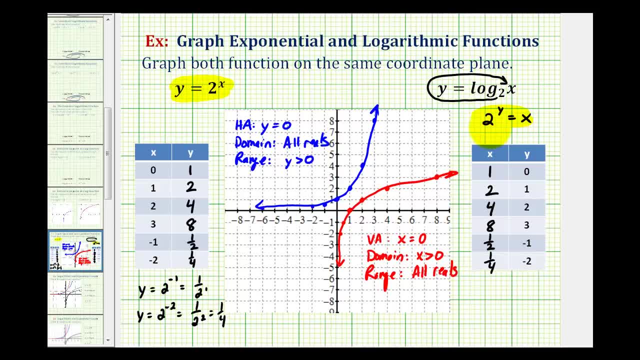 have been interchanged, as well as when both equations are written in exponential form. Notice how the exponential function has a horizontal assin tot of y equals zero. The log function has a vertical assin tot of x equals zero, And notice how the domain and range have also been. 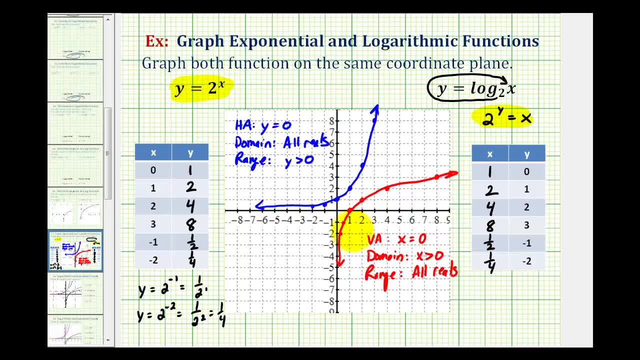 interchanged between the two functions, So we should recognize that these two functions are inverses of one another. Another way to show that these two functions are inverses is to graph the line y equals zero And y equals x and show these two functions. 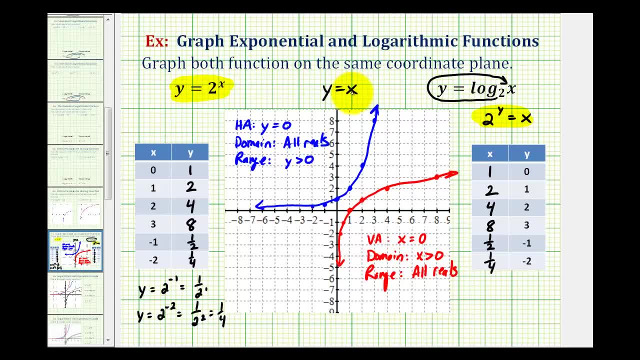 are symmetrical across this line. Well, this line has a y intercept of zero and a slope of one, so it would pass through these points here and look something like this: So notice, if we folded these two functions across this line, they would match up perfectly. again showing: